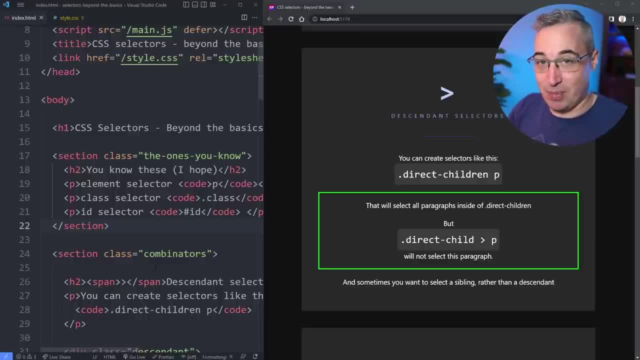 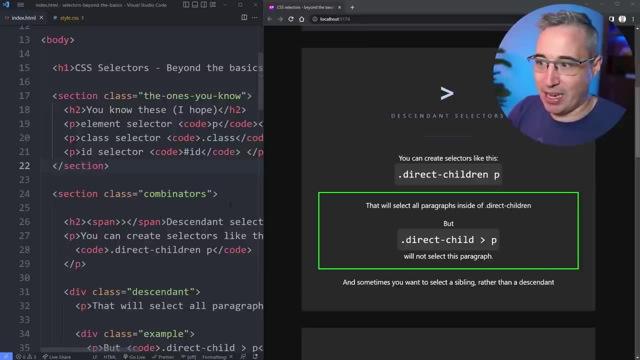 This is by no means going to be an exhaustive. I want it to be things that, from a very beginner level, you can sort of take that one next step up and do things from there, And the first thing we're going to be looking at is a couple of combinators. 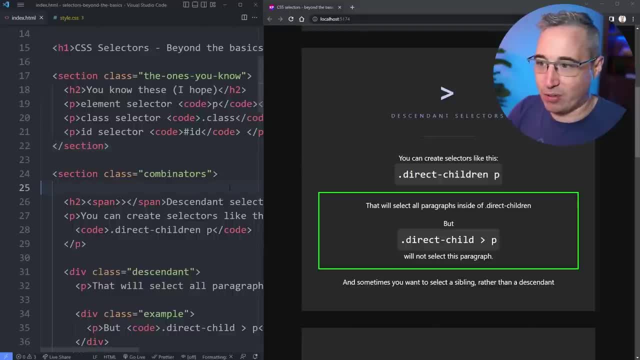 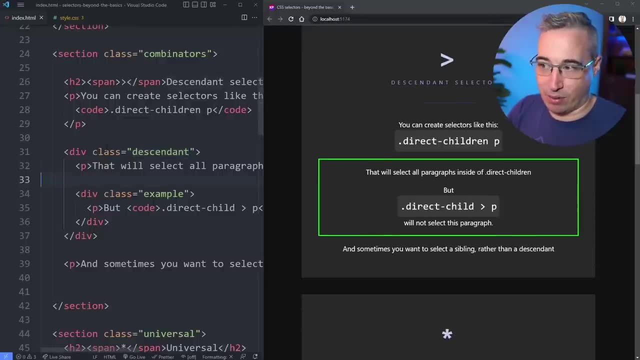 and there's some more advanced combinators you can definitely dive into, but I want to look for now at the descendant ones, And so here you can see, this green box that I have set up right here is called a descendant. It has the class of descendant on it and I put that on there. 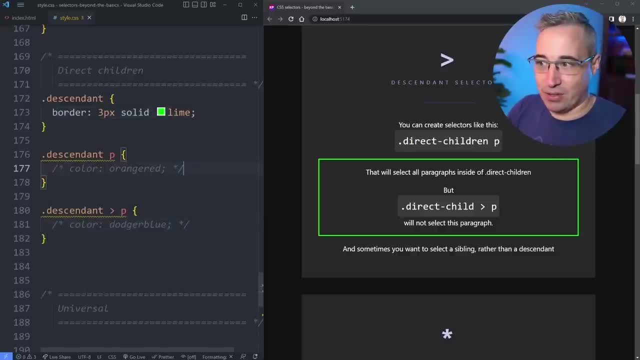 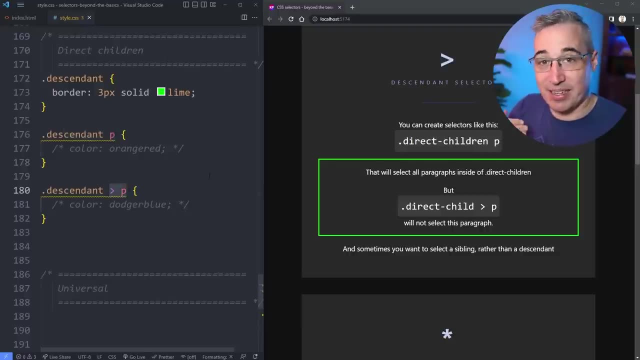 And we're going to jump on over to my CSS And here. first, we have two different types of descendant selectors. The first one here is a general descendant selector and the second one here is a direct child selector. So they're a little bit different from one another. 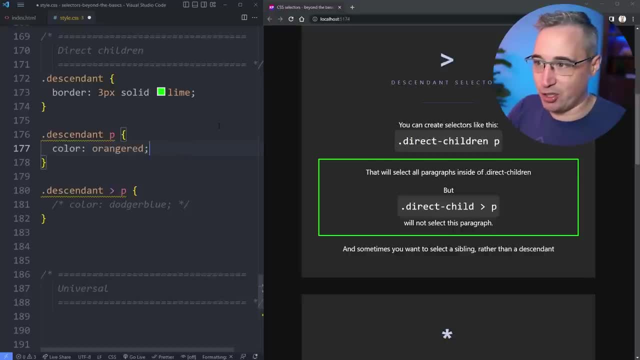 even though often they can actually seem very, very similar, especially early on. So what I'm going to say is I'm going to choose all my paragraphs that are inside the class of descendant and we're going to switch their color over to orange-red. 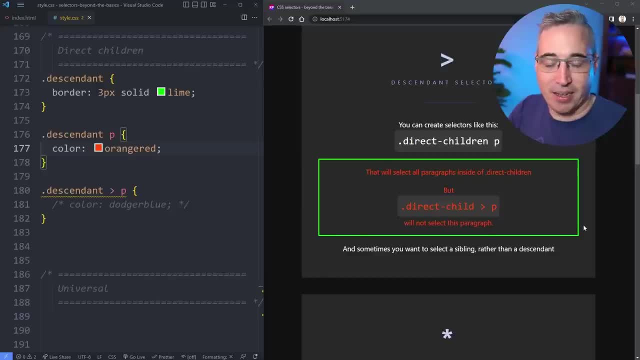 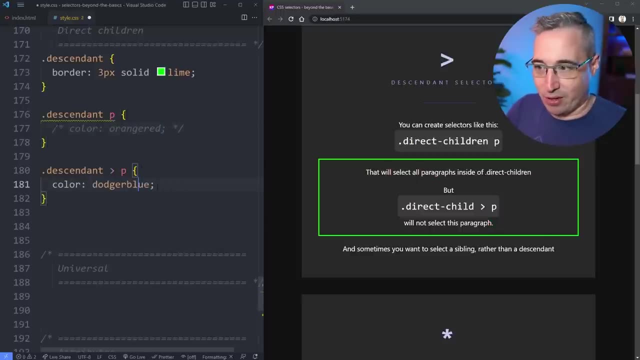 And you can see all the paragraphs. so all the text that is inside of there has switched over to be the color orange-red. Now let's turn that one off and let's come and take a look at this one and turn that one on and hit save. 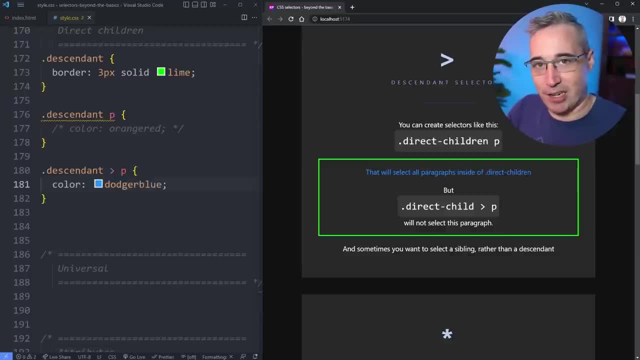 And you'll notice, it's only this first paragraph now that has actually changed and none of the other ones have, And the reason for that is is we're only looking for paragraphs that are a direct descendant of my descendant class. So, coming here, this paragraph is a direct descendant. 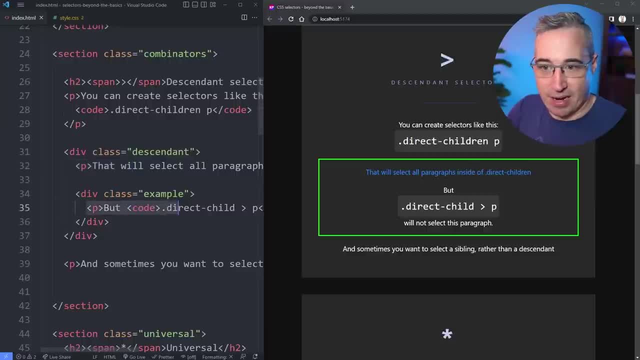 so it's the child of my descendant one here, Whereas this paragraph and everything that's over here is nested inside of another div. So because it's nested inside, it's not a direct descendant. it goes a few extra steps in. 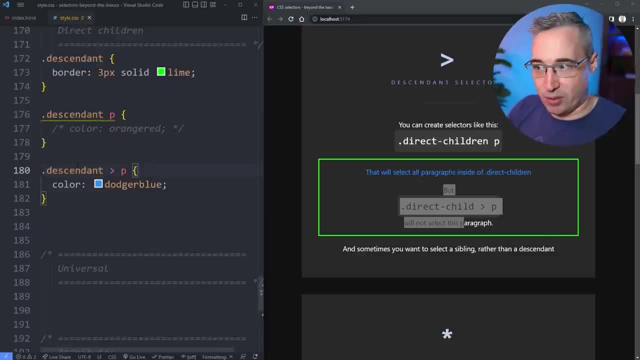 and it's not selecting it. Both of these can be very, very useful: This one when you want to be more specific and choose something that's only the direct child, whereas this one if you need to select all the children. 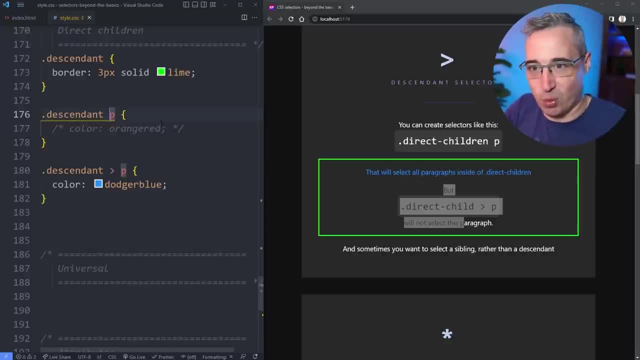 or all the children of a certain type, then it can come in handy as well. Now a word of caution on descendant selectors like this. some people do not like them because they raise the specificity of what we're working on, And if you're not really comfortable with specificity, 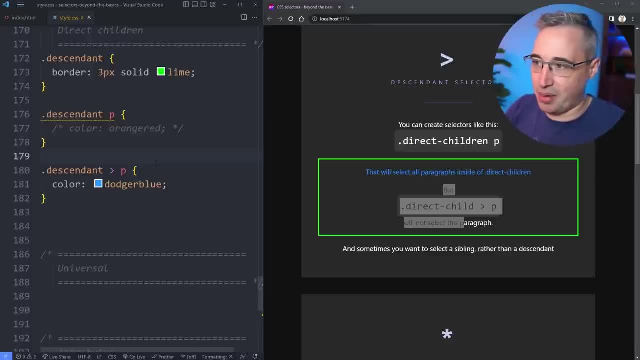 I'm not going to deep dive it now. I have another video, and I'll remind you at the end about that. It's a very important concept with CSS, though, and what that means is, say, I came here and I said all my paragraphs should be the color red. 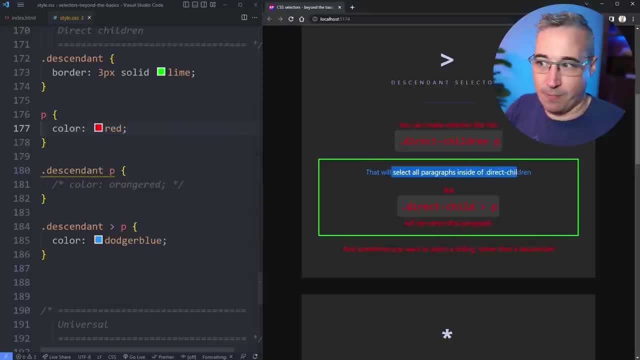 and you can see they've changed over to red, but this one is still blue. And this isn't based on the order of them, because if I bring that down here, it's still blue. So it's not the order, it's the specificity. 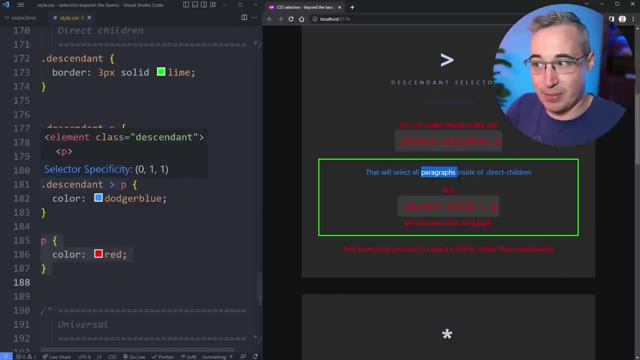 And if you're using VS Code you can hover over a selector and it shows you the specificity of it. For here we have a 011, because we're combining the paragraph with the class selector here, so it gives us higher specificity than a simple paragraph selector. 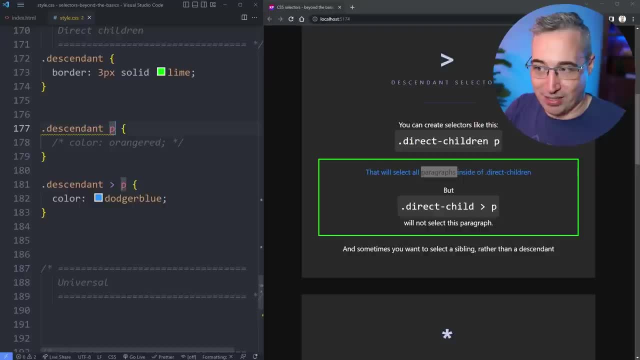 Some people really don't like that. I think as long as you're not going too crazy and selecting like paragraph and then span and then something else, then you can probably get away with it and sometimes simplify your code a little bit by using them. 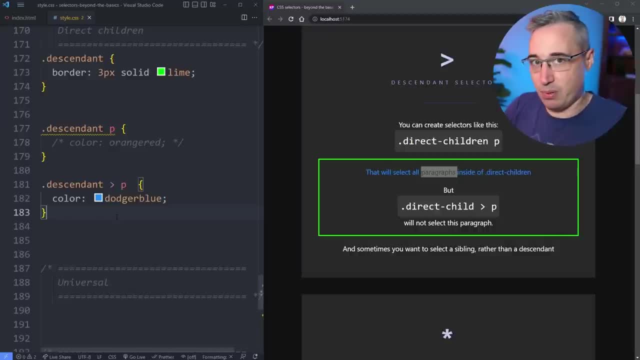 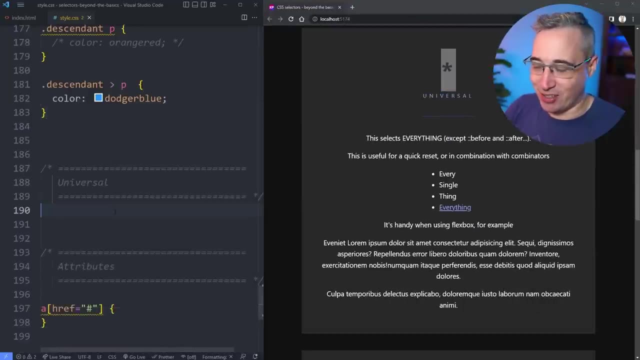 But just do be a little bit careful. if you do use it and know that some people prefer not using them at all and just using class selectors for everything, Next up, if we come down, is the universal selector, which is just our star. 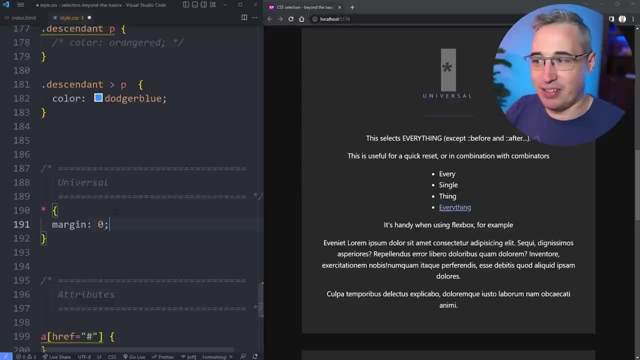 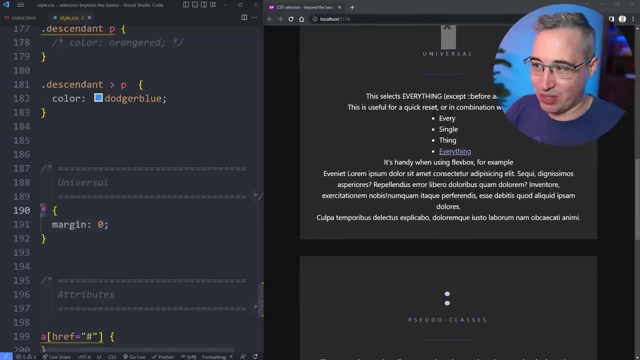 So let's come down here, do star- and this is really common to see- resets that do something like margin zero and just eliminate the margin and everything. Goodbye margins. So we're just selecting every single element on our page and applying a property to it. 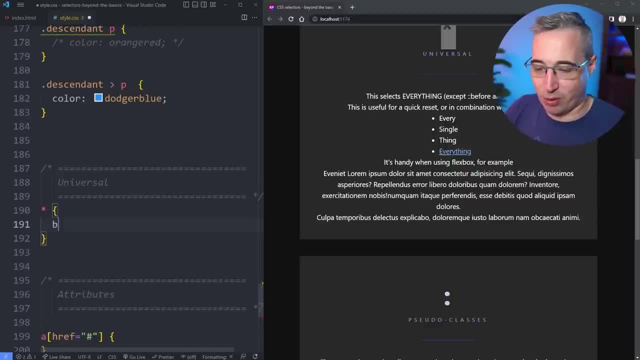 Now one thing with the universal selector- or this is very popular: ordering a box, sizing, border box. This selects every element on our page, except for pseudo elements. If you don't know what those are, we're going to cover them. 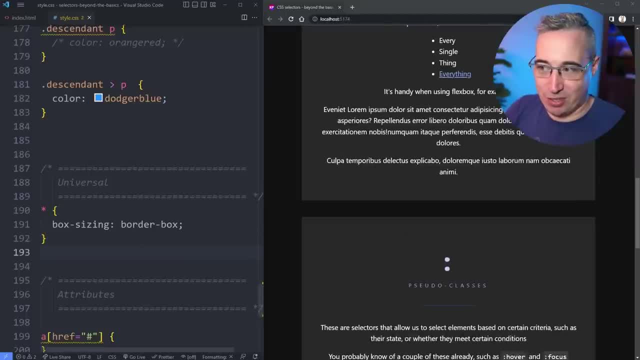 That's one of the things that we're going to look at in this video, But just know that those are sort of common things that we see or common resets that you'll see, and they're on the star selector, which actually has a specificity of zero. 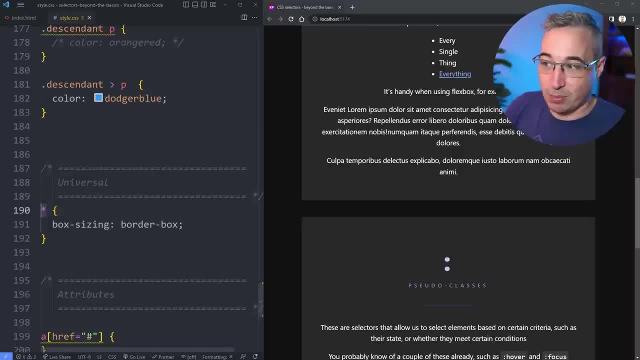 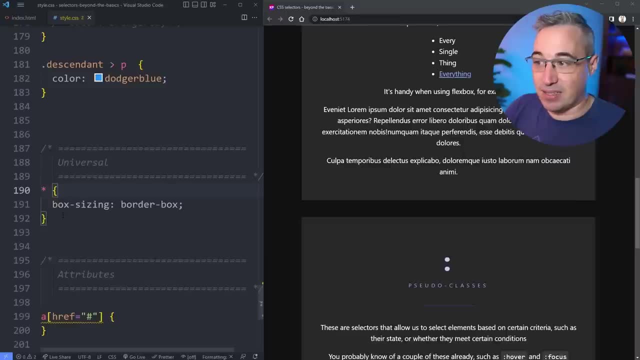 which also makes it very easy to overwrite. The one thing I would not put on this is any of the font properties. If you're doing your font family or you're doing a color or other things like that- font size, line heights, all of those things. 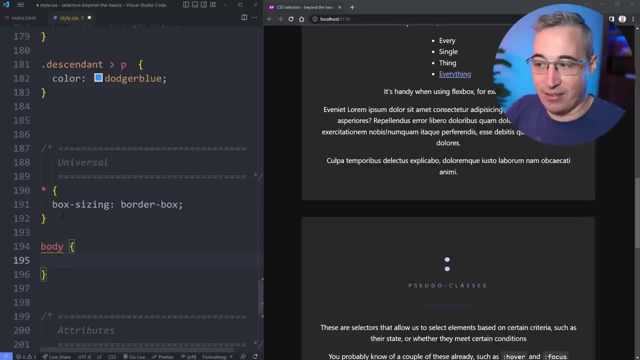 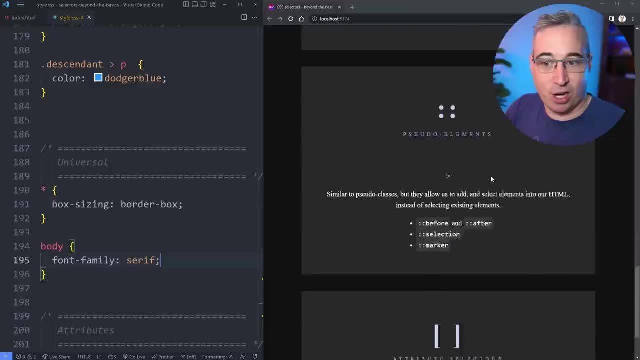 you can do those on your HTML or on your body. If I say body and do font family and then here do a and then do the serif, it's changing all of my fonts over to the serif already, because this is relying on inheritance. 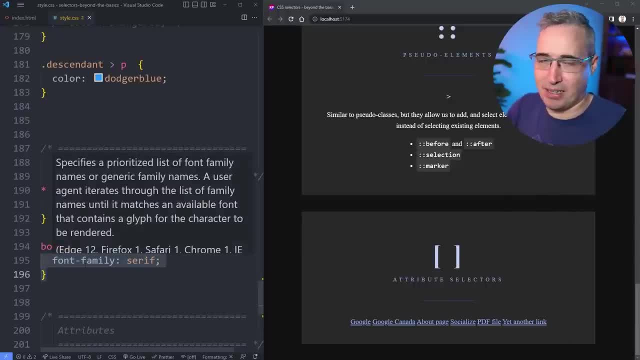 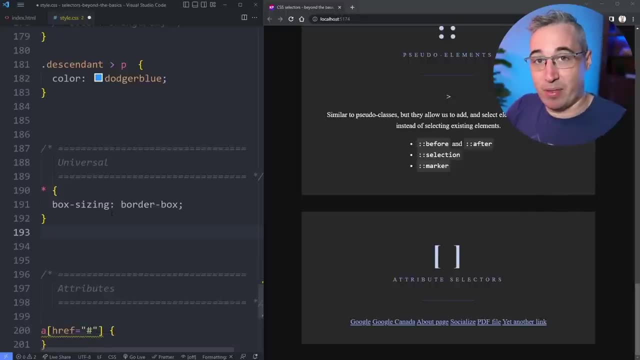 And so it's better to place things that are inherited- and that tends to be all your font properties- on your body or on your HTML element and then just rely on inheritance. But for things like margin, where they're not inherited from one to the other, 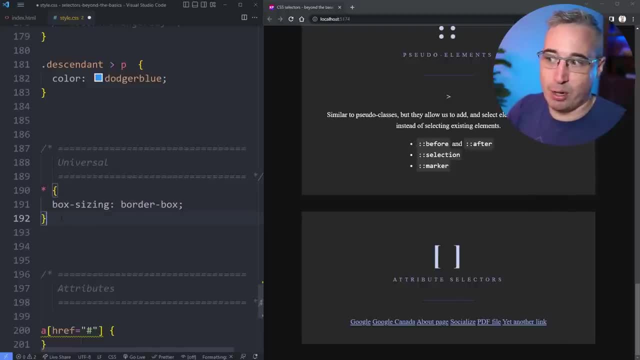 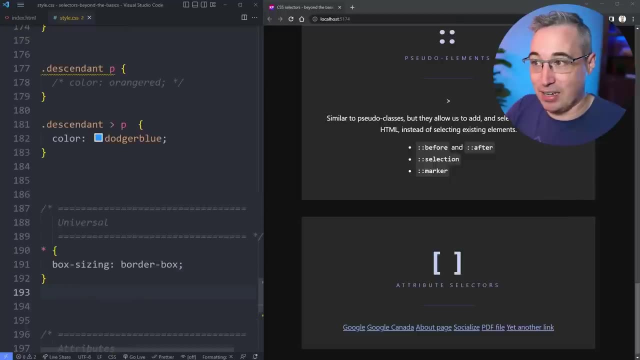 your margin, your padding and other stuff. that's where it's quite common to see those reset with the universal selector And of course you don't have to use that to select everything. You could use that in combination with these, which could also come in handy sometimes. 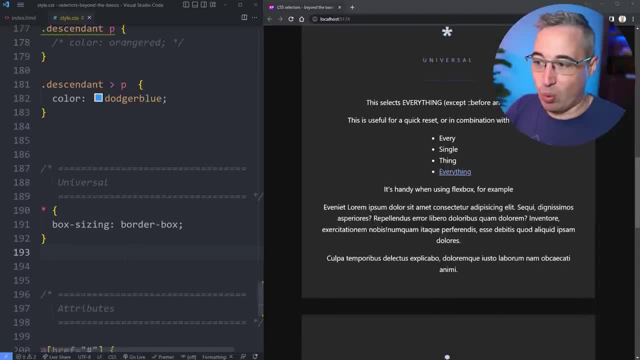 So we're sort of skipped ahead because of those margin shifts. But one time you'll see that and I don't want to get too advanced. but let's just come here and if we go down you'll see I have this even columns class. 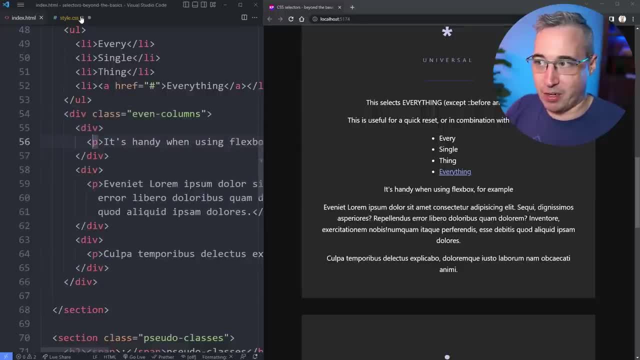 So, on that even columns class that I have right here, I actually want to make some columns And I don't know how new you are, but let's select that. We'll do even columns, and maybe you haven't got to flexbox yet. 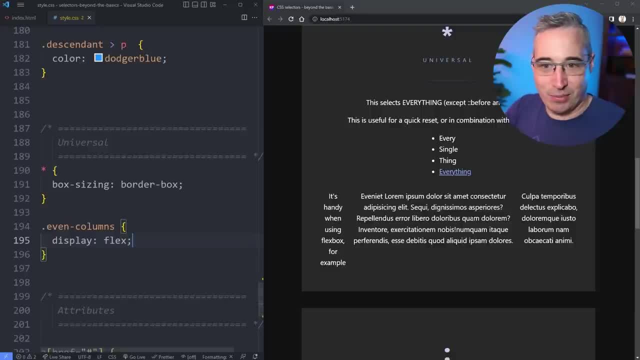 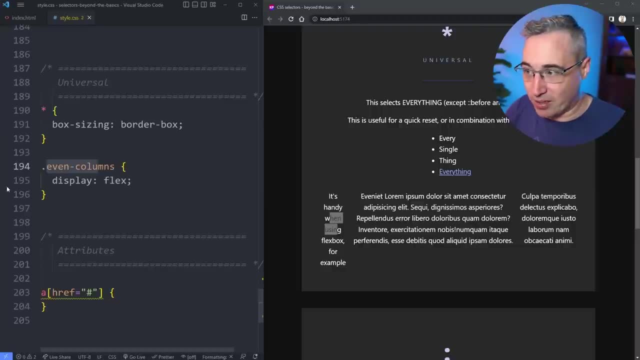 but we're going to throw a display flex on here anyway And we're going to see that we actually get these different sized columns coming in Coming from here. they're definitely not even columns And with the way flexbox works, which is a layout tool, 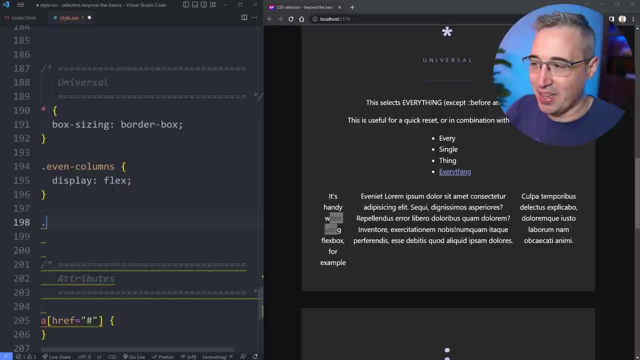 and if you haven't learned it yet, definitely will be something you're learning soon. But a common thing to do would be to do even columns and then choose all the direct descendants. So we're saying, only if it's a direct descendant, we're not doing this. 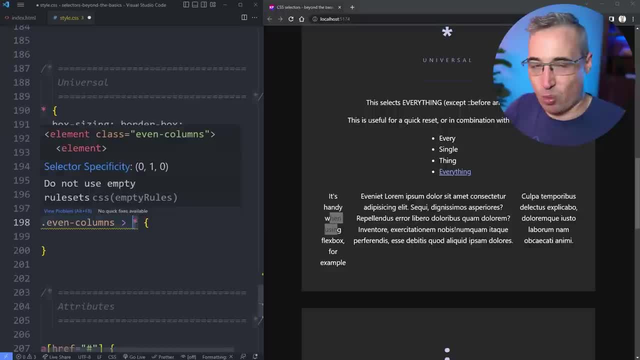 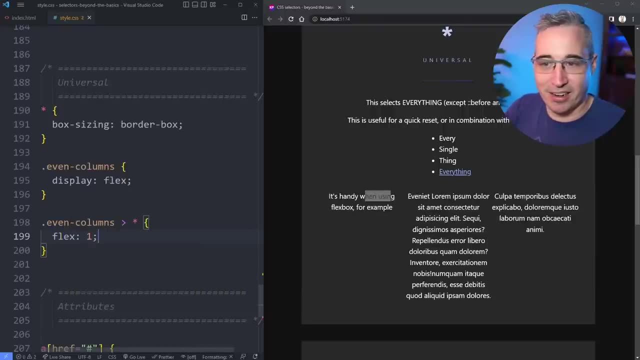 but only if it's a direct descendant. we're going to choose it, no matter what it is. It could be a paragraph, a div, an article, whatever- it doesn't matter- And then we could do a flex. Again, I'm not going to deep dive why I'm doing this exactly. 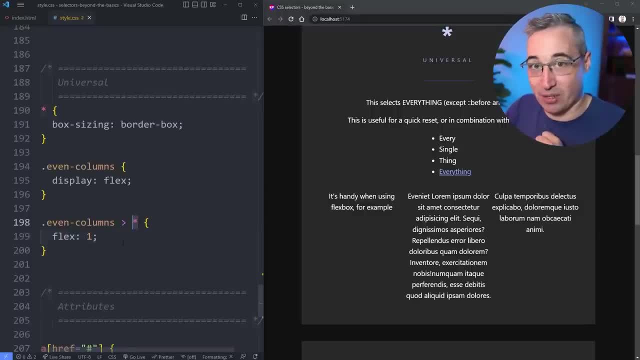 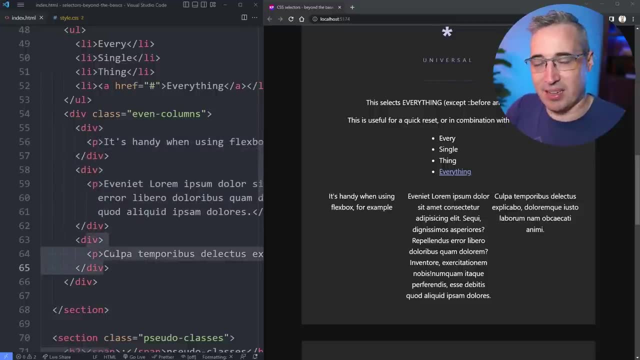 but just to show you like sort of a other example of where the star selector can come in handy right there. So again, we're selecting all the direct descendants. So this div, this div and this div and the flex one is basically saying they all have to be the same size. 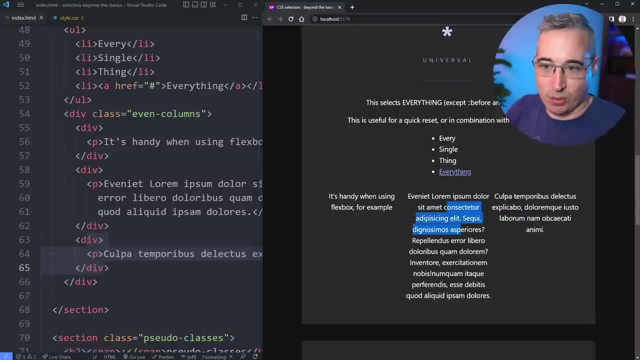 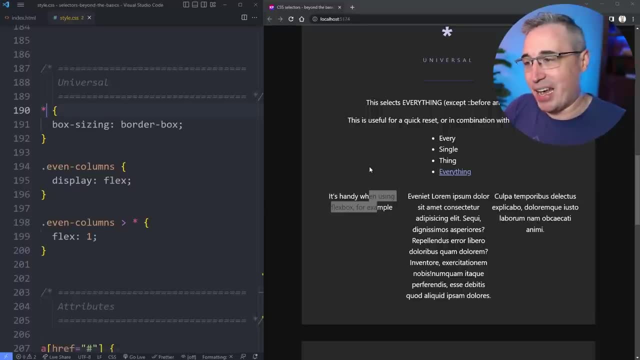 and behave in the same way with their growing and their shrinking, which makes it so we get three equal columns. So yeah, a couple of use cases there for the universal selector, And from there let's move on to pseudo classes probably already know your hover and your focus. 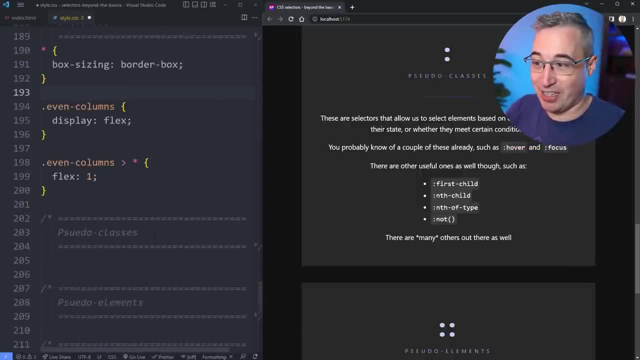 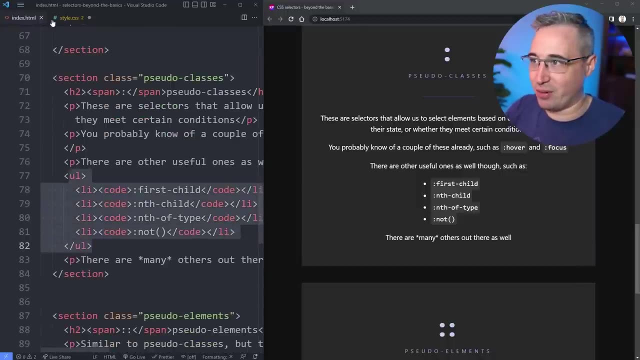 I'm sure you've come across something with those already, but just in case you haven't, let's move down to here and let's go and look at what we have in this area to play around with. So let's just go on this UL that I have right here. first of all, 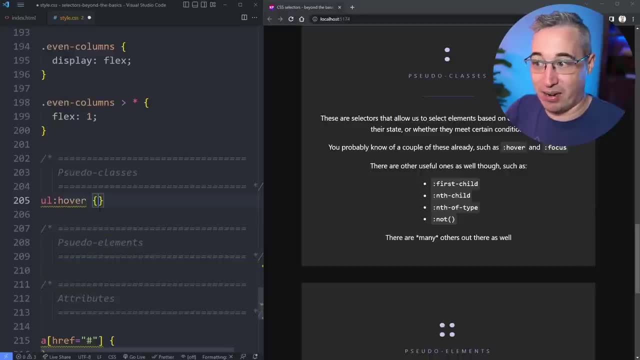 and we're going to choose that. So I'm going to say the UL and we're just going to throw a hover on there and say that the color is going to be red and hit save. So now, when I hover on top of the UL with my mouse, the color changes to red. 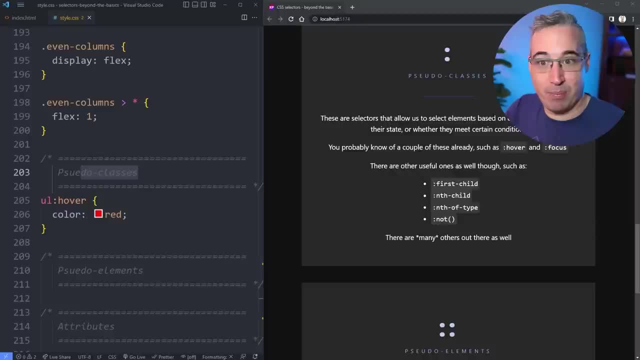 So in general, pseudo classes are very good based on different states or different criteria for the element. So another example: hover is not really the practical one for a UL. You probably want to do this on a link And if you're doing links you should also include it's very common to see your A. 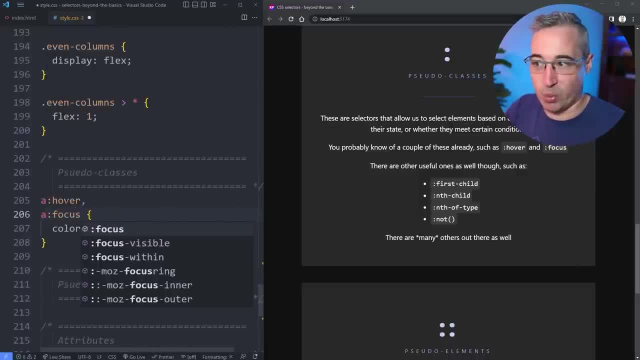 You'll have your hover and then you'll also have an, A focus on there as well. So we're selecting both of them and doing the same style. So, whether we're using a mouse to select it or keyboard navigation, where you can tab through links, then the both of them are going to have. 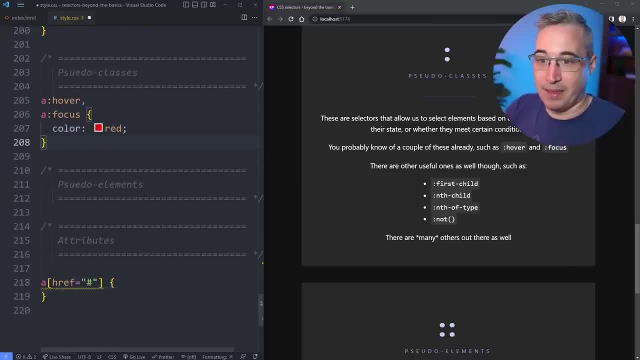 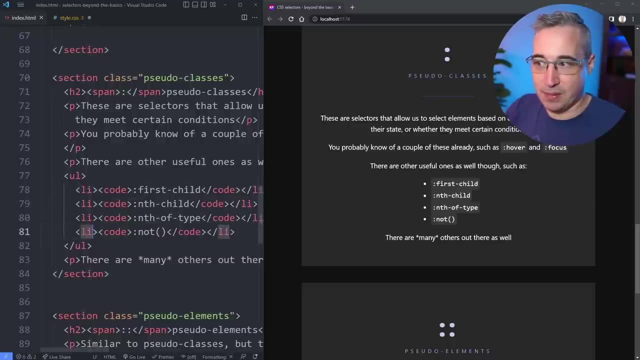 the same state on there where they're both changing over to red, If we go to that UL again, or actually, let's not do the UL, Let's look in the UL. We have these allies, So looking at that, let's choose. we can just do all of them for now. 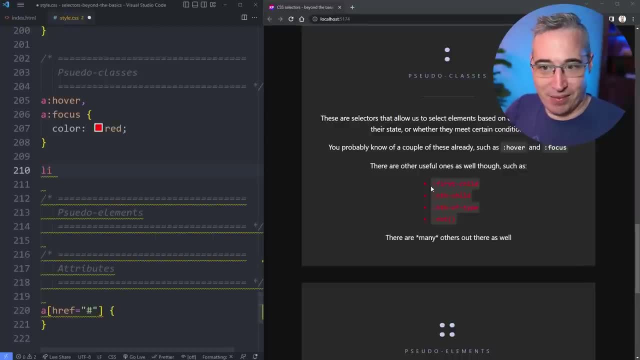 It's fine. So we're going to say the ally And then, as you can see here, I've listed off a few different ones. Let's save that so it stops updating. So, on the ally, we could choose different, as I said, different states like hover or. 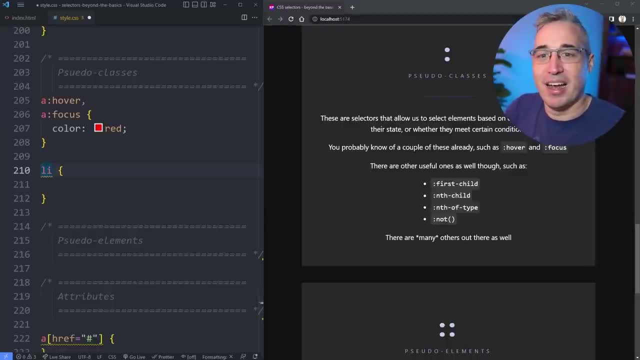 not hovering or hovering. I guess we're not doing a not hover, but we can choose something, also based if it meets certain criteria. So we could do it if it's the first child. So let's do that. First child is going to be a color of red and then only the first child becomes red. 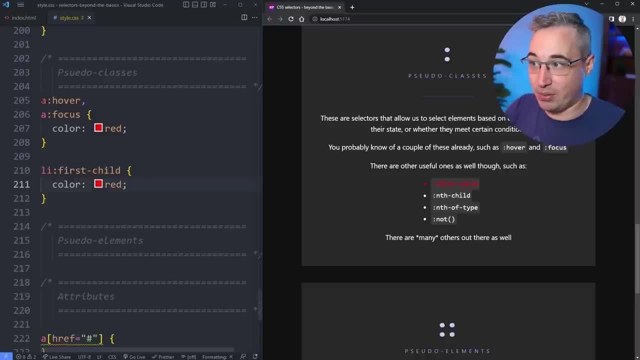 Of course you could do this for other things that could be useful. For example, one place you'll see it used sometimes is on paragraphs. So you might have like article P, first child, or maybe it actually be of type: There's first child and I didn't put it in the list, but there's first of type. 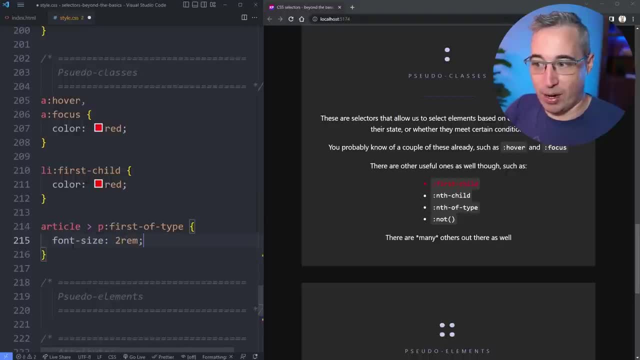 And then on that the font size could be like a two rem, And so in a regular article that you might have on your page, the first paragraph- it's like the introduction paragraph- is actually bigger than the other paragraphs And you don't have to go and add a class to where you need to do that or something like that. 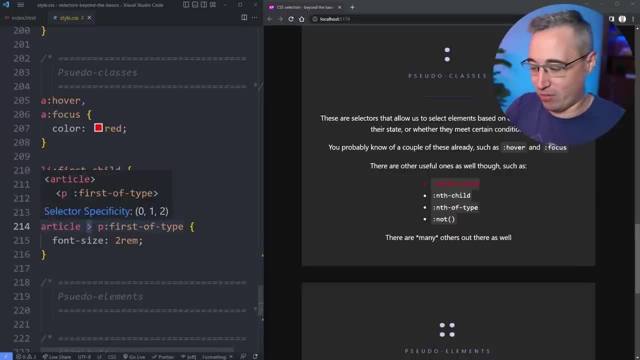 We can select it using our direct child combinator, or we could do that as well, but it's a little bit more dangerous. So the direct child combinator with our paragraph only if it's the first paragraph inside the article while it come into effect. 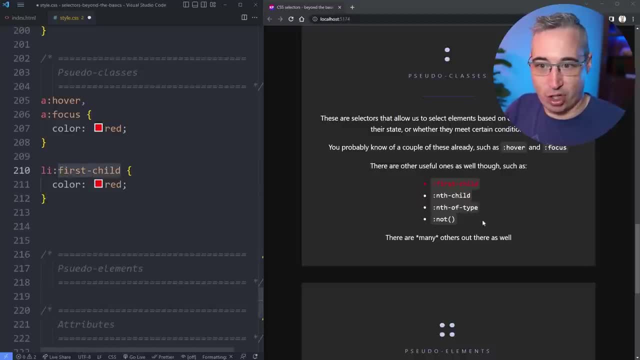 So that could be something useful right there. The other one, other than first child that we listed, is also nth child. Nth child. I could do a video just on nth child. It can be very. I could say nth child too. We'll start there. 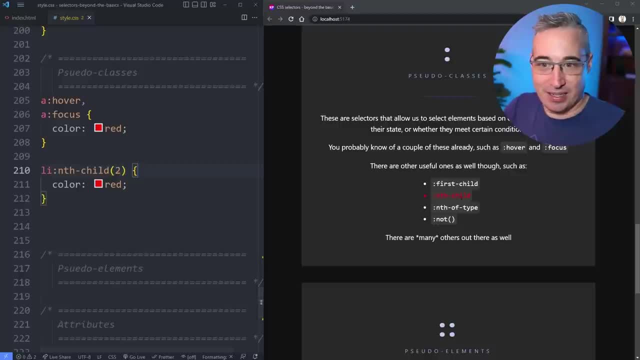 Whoops, not nth child, Sorry, And you'll see. it's selecting the second one. or I could do three and I could save, or I could do one and I could save, And this does not work like other programming Languages that start counting at zero. 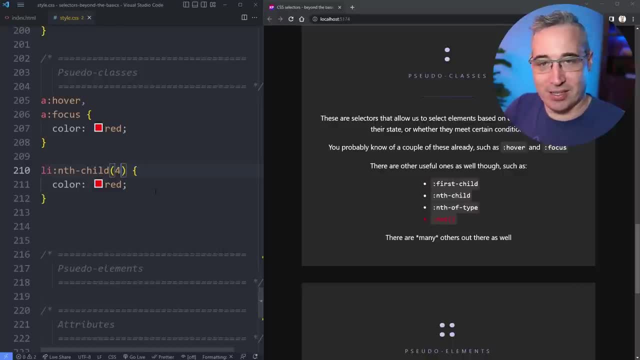 This starts at one, So you just say which child you want and you can select things that way. Alternatively, you can do like a two n and it's going to select every second one, or I could do a three n. We're not really going to see it work here. 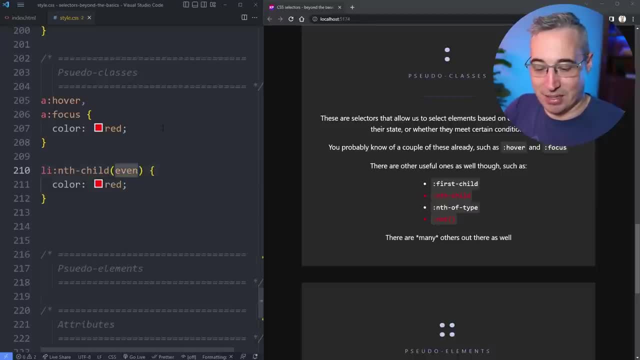 You can also do even and it's going to select the even ones, or I could select all the odd ones and do things that way as well. And you don't just have to be doing color. You can be doing backgrounds if you need, like a zebra pattern on something on a table or something like that. 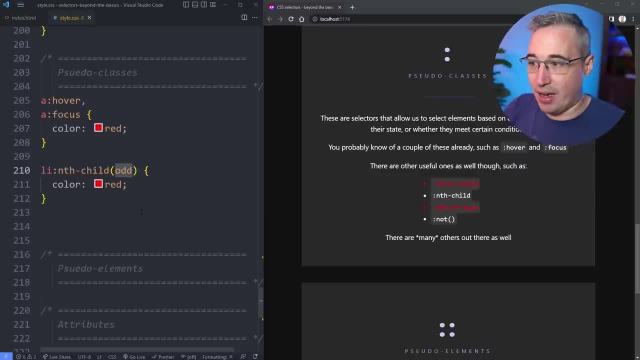 So there's different places. you might want to use an even or an odd, Or, as I said, you can do a three n and it's going to choose every third one. or you could choose every fourth one and you could do a lot more. 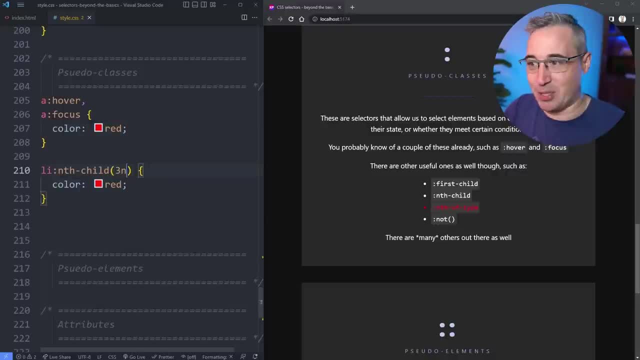 I'm just covering the very basics of what we could actually do with nth child. So an interesting one there. Let's just put this to two: n for every second one Even is a little bit easier to read. So whichever one you want, they both work fine. 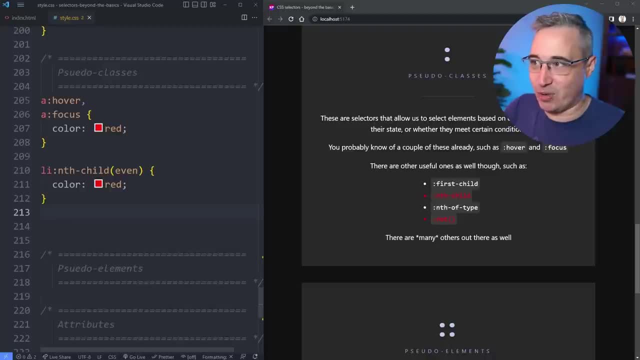 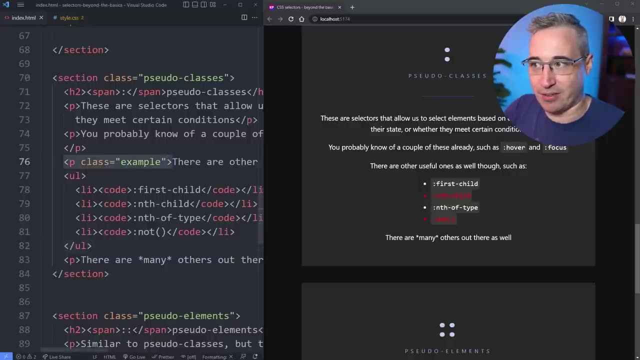 And the last one I did there is the not, and not is an interesting one, And for not, let's jump back over to my HTML file for a second, where I've set up this paragraph of example here. So we're going to go. 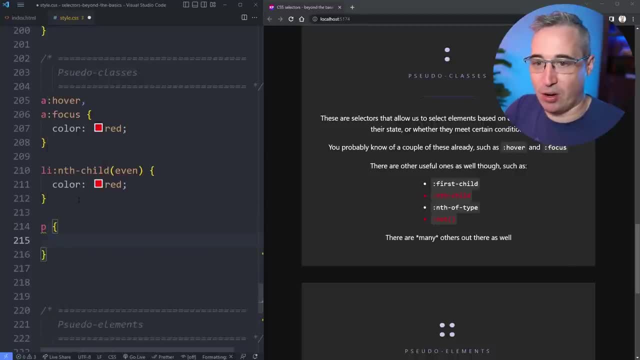 And we're going to select all my paragraphs first. We're going to say: paragraphs are all going to be color And let's do my lime like that, So all my paragraphs are getting a lime color on them. But what we could actually do here is not dot example. 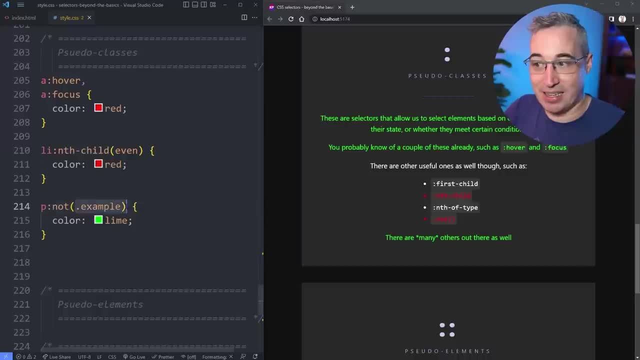 And now it's selecting every paragraph that does not have the class of example on it, So we're not selecting this one here. Kind of cool, right. You can actually combine that with like nth childs that are in here as well and other stuff and get kind of weird with it. 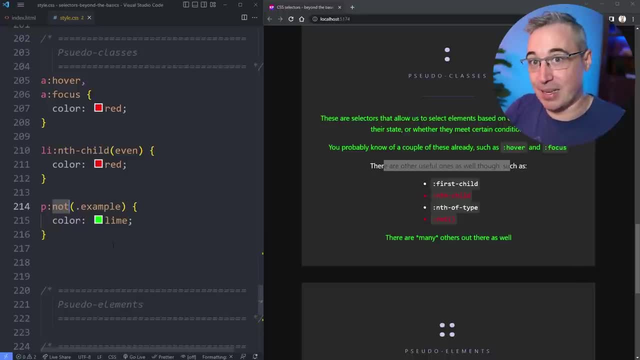 But the not one can be very, Very useful if you need to select a lot of things except for something very specific. like you're selecting all your links, So you're doing a, but not your like nav link or something like that, So you want to select every link that's on your site but not your nav links or there's different things where it could sometimes come in handy. 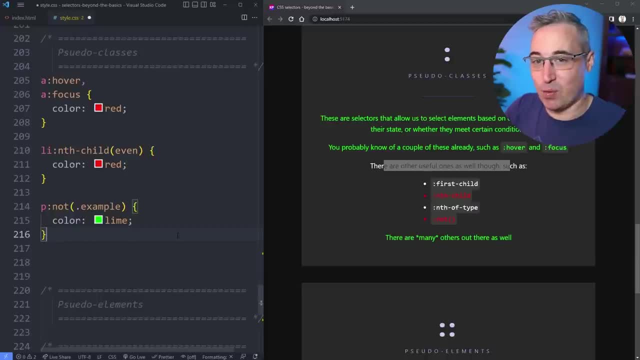 So the not selector, it's one of those ones that you might not see immediate use case for. But then you're going to run into a situation where you're like I wish I could do this but not select that, And then hopefully you go wait. 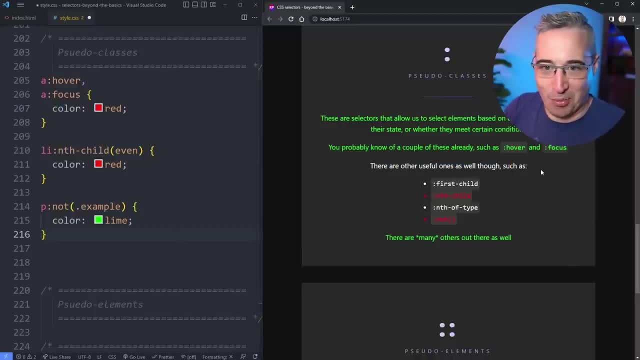 I can Select something and remember to look up how it works. So, and a lot of CSS is not memorizing all of this stuff, It's just knowing it's possible and then looking it back up after. Don't feel like you need to memorize all of these, because this is just scratching the surface. 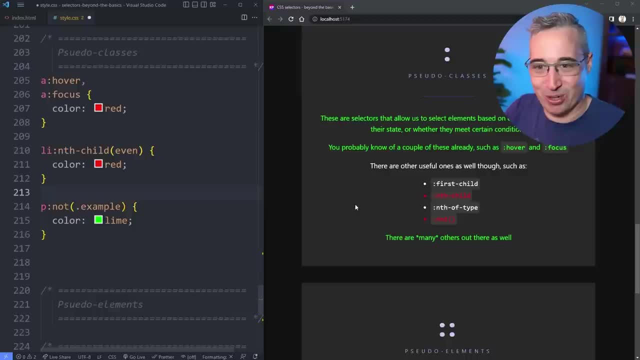 There's so much more. It's one of the reasons I love CSS is because there's always more to learn, But not everyone is always as enthusiastic about it. but you do not need to memorize all of these things. It becomes very repetitious. 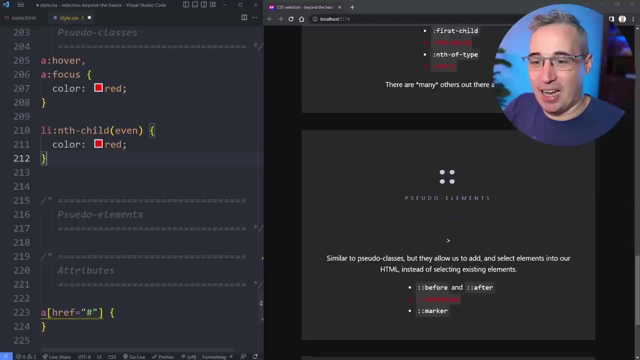 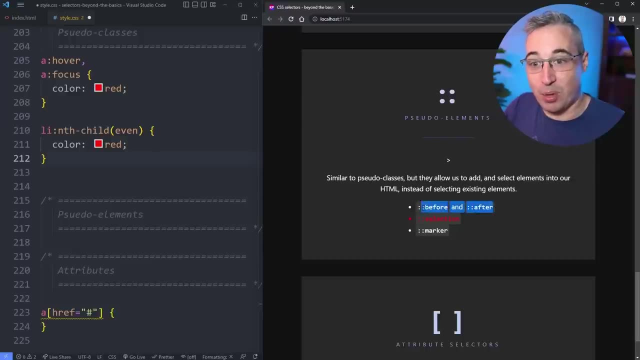 These things start to sink in, So don't worry about it too much. Another one is pseudo elements, And there's a before and after that I'm not actually going to talk about in this video, but they're very common ones that you're going to see. 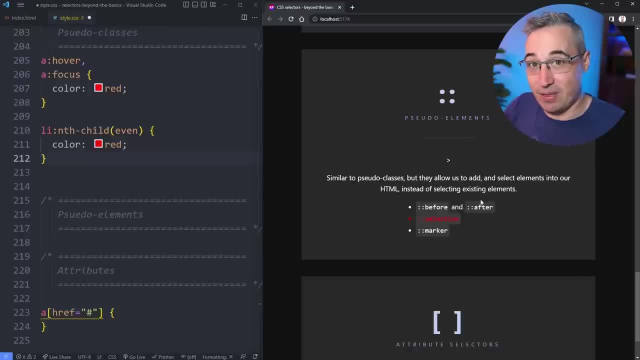 And the reason I'm not going to talk about them right now is because I've deep dive them, So I'm going to put a link to the video in the description and another one that I'll remind you about at the end, just because I could talk about them for a really long time and they're kind of specific in how they work. 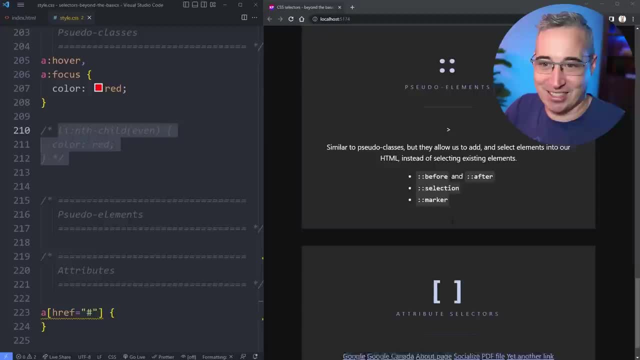 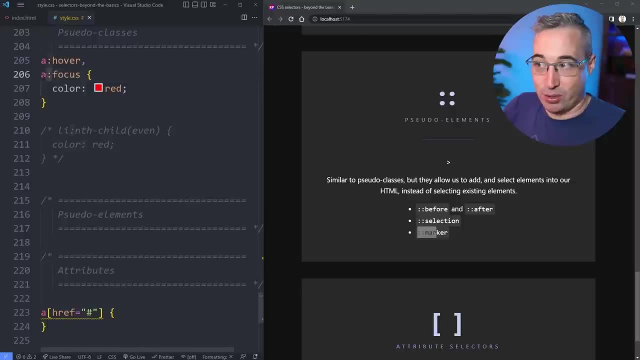 But let's turn this off because it's changing our list right there. But the ones that I will look at are the selection and the marker. Pseudo elements actually are very similar to pseudo clients: Pseudo classes with pseudo classes. we have the single colon with a pseudo element. 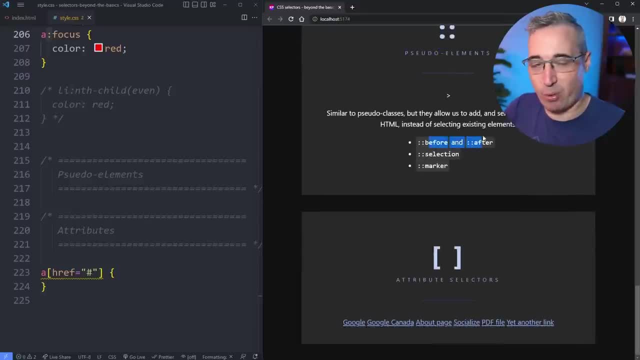 It's just a double colon instead, And especially with the before and the after, they're like injecting extra elements into the Dom and it's basically letting us select new elements that weren't previously available. in a way, or it's sort of different states, but in a different way than pseudo classes are. 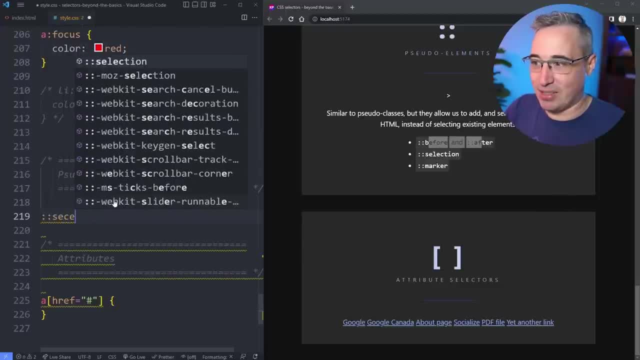 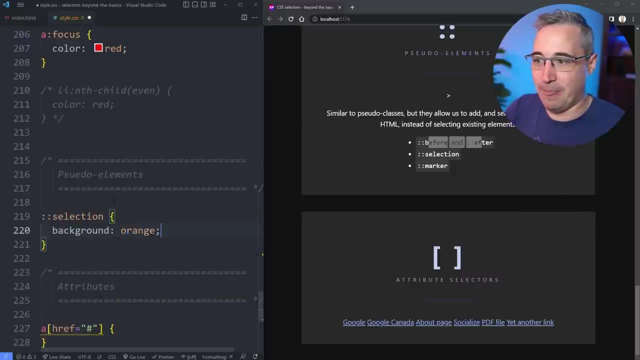 I don't know, It's a little bit weird, but we can do a selection, pseudo class, So selection. you got to spell it right. And let's say we're going to set a background on here. I'm going to go with the color of orange and it probably won't look great, but now when I select stuff, the background color is orange instead of what was the default before. 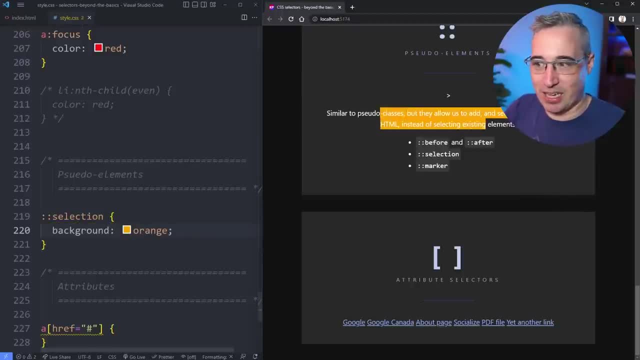 I don't even know it was this blue color. So instead of the blue color, we can change that. You could change other stuff and you can't change everything, but we could change the color over to black and we can customize the selection, which always makes a nice touch on a site when you're playing around and doing something, to have the selection color fit with your color scheme. 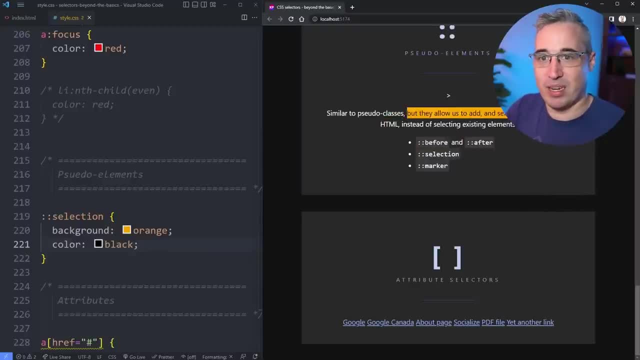 Just make sure that the contrast with the text is high. Often we'll select something as the reading it, or they might select something You want to make sure when it's selected it's still easy to read. But, as I said, you can't change everything within this. 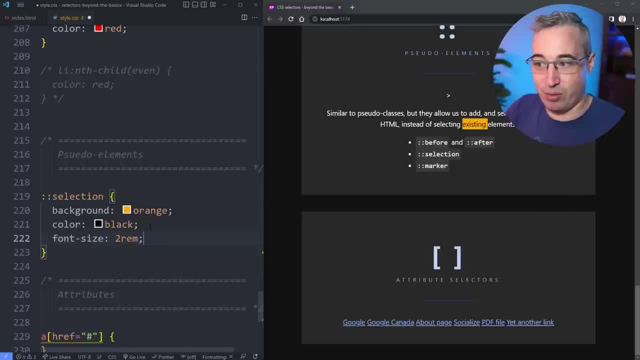 There is a limited set, So if you did something like font size here they would break stuff, so it just doesn't work. So you're not changing font sizes or getting too crazy, But just for changing colors and doing other stuff like that it can look kind of nice. 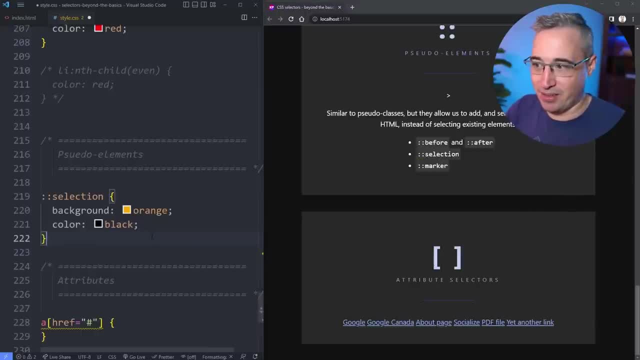 And another one is the marker here, because see how I have these bullet points. Well, let's say I have my ul and I could say marker, and I could say color is purple. let's say this time purple, and oh, it's not ul, it's li. 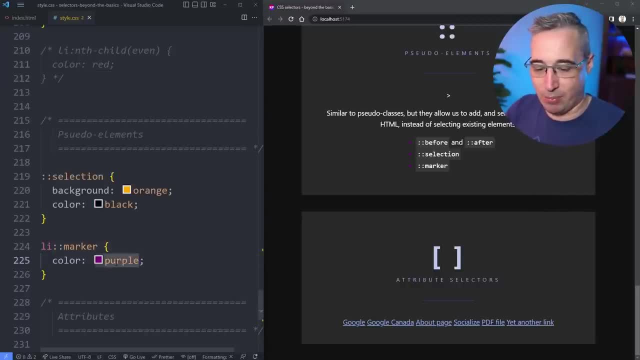 Sorry, And you can see I've changed those over to that And I think plum would actually look a bit better. Let's switch that over to plum and I can change the marker of my li's. So the bullet points and the numbered list. if it's an ol, those are called markers. 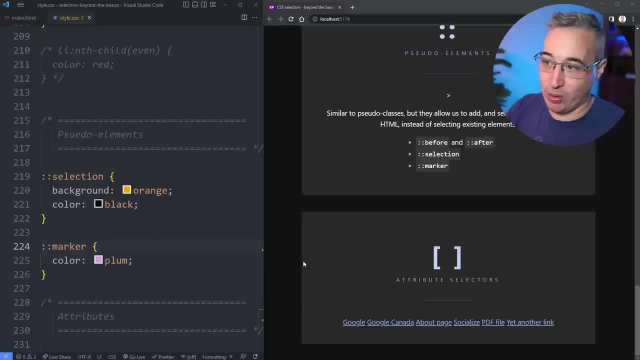 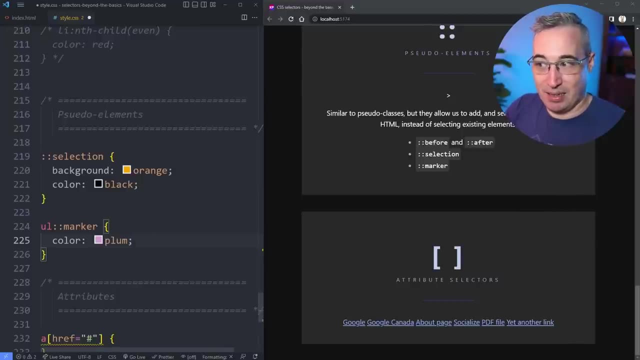 I could change all of them just like this, and it would do my ul's and my ol's, or you could specify one or the other by just including that at the beginning of it. And, interestingly, if you're doing an on ordered list, like we have here, you can also change the content of it. 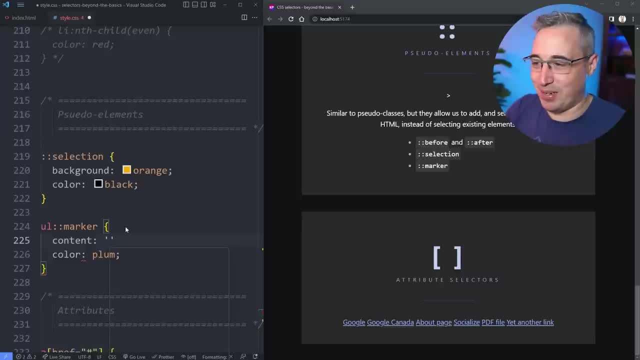 And let's put in an emoji here. So I forget the shortcut, but I have a custom key set up for it. But let's just come in and put the fire symbol or fire symbol emoji there and turn off the color. That should work. 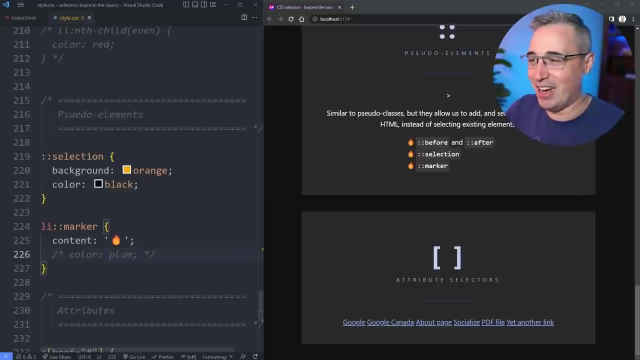 Oh, I did ul again, li, That should have worked And maybe something like that. So you're not changing the content of an ol. So we're using our direct child combinator again to make sure we're only looking at the ul's and you can. 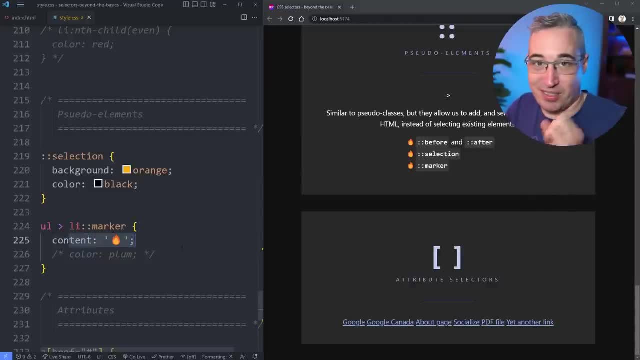 actually change it with this content there to something other than just the simple dot. if you want to and play around, change the colors, do other stuff. This is another one that is limited in what you can change. You can't do anything you want to it. 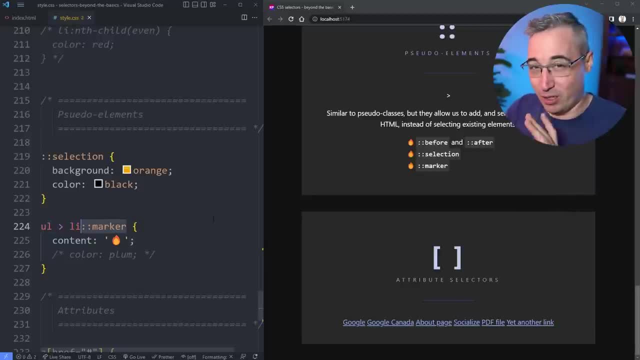 but you can do font sizes and play around with other things, Though if you go a little bit too crazy it can be hard to align stuff properly and everything after that. So see it as like sort of limited changes you can make and not something that's a little bit too crazy. 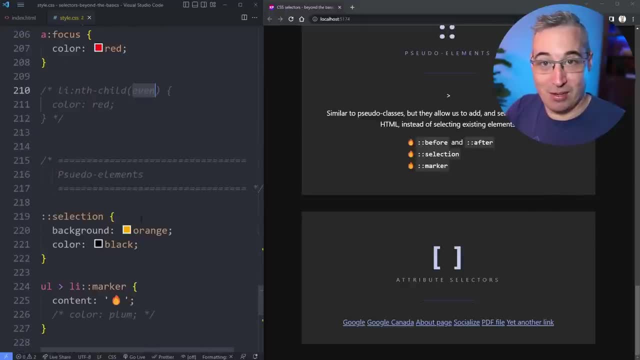 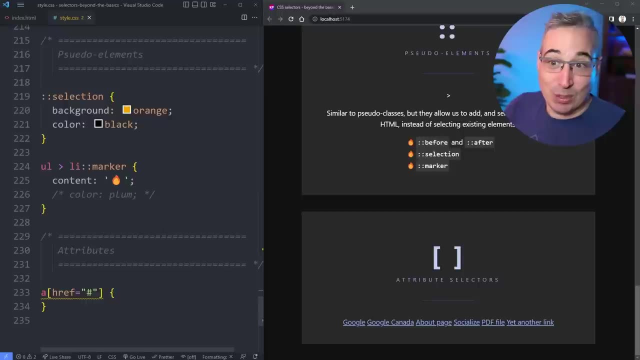 And this could be fun for a bullet list combined with your nth childs- and changing. start cycling through different icons and stuff if you're looking for ways you can practice, And the last one that we're going to talk about is our attribute selectors, And what I've done is I put all these links down here at the bottom. 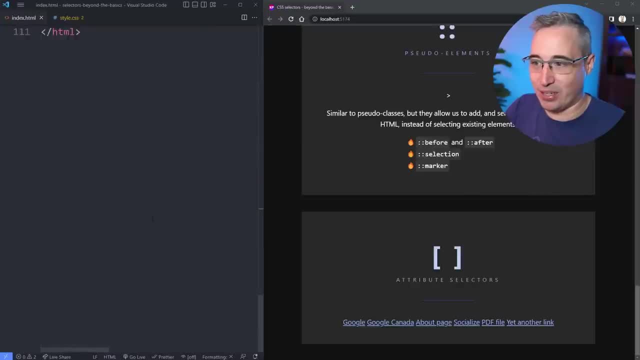 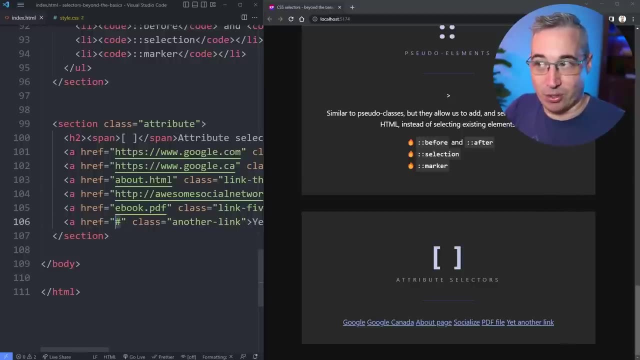 and I have this Ahref of this. So if we go and take a look at all the links we have down here, they all actually are going somewhere, but I forgot to put this one and I forgot to tell it where to go to. 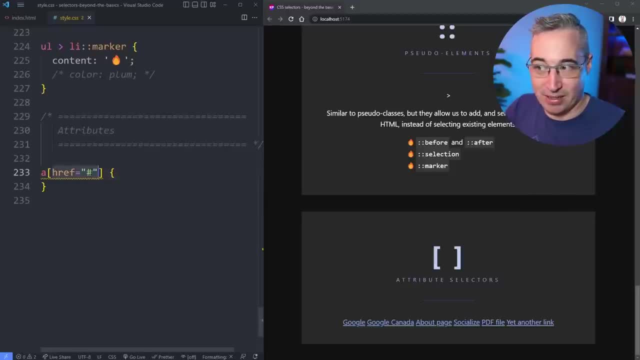 So this is really interesting where I can write: the entire Ahref is equal to that there. So I'm selecting the Ahref attribute that is equal to the hashtag, and I could say: color is red and only that link is going to get changed. 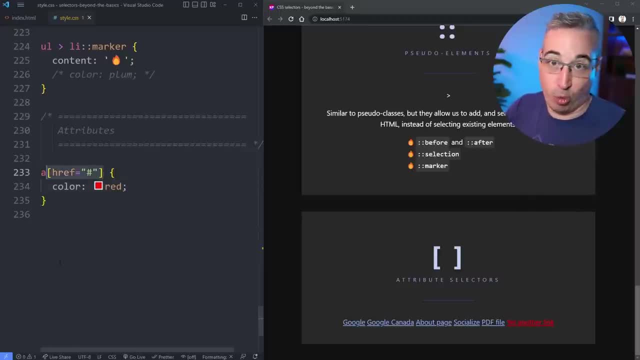 rather than all of them, because it's the only one that has an Ahref going nowhere. So a little like warning symbol, like watch out, this link isn't going anywhere yet. So if you did like a personal project where you had some blank links, that you were 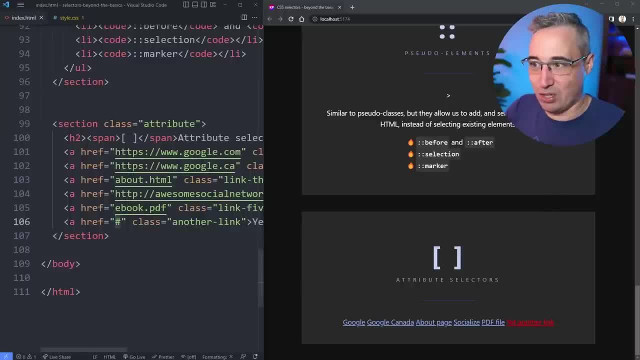 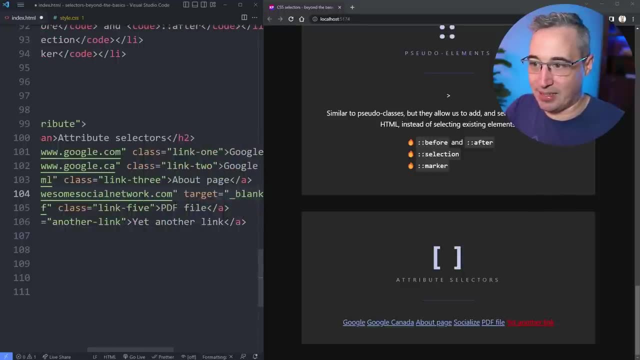 going to fill in later. it could be a good way to catch them, And of course you could do other stuff on here too, Like all of these have classes. but let's say we take off link four here, so all of them have classes except for this one right there. 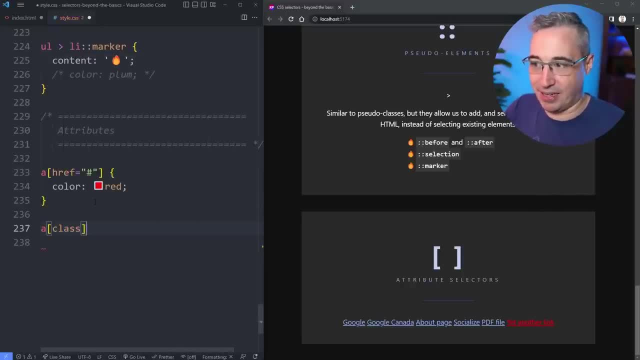 So on. here I could actually say a class, and it doesn't matter what the class is, Color is going to be, we'll go with plum again, I guess plum, And you can see they've all changed. Why are they all changed? 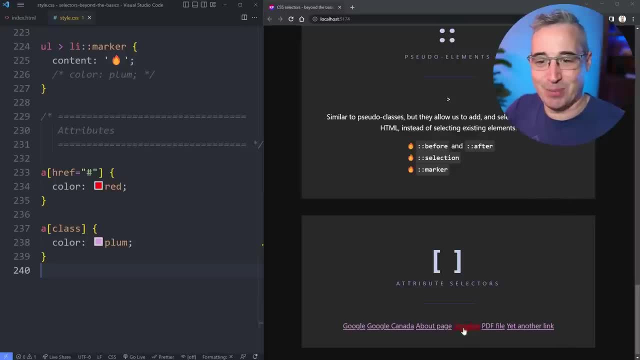 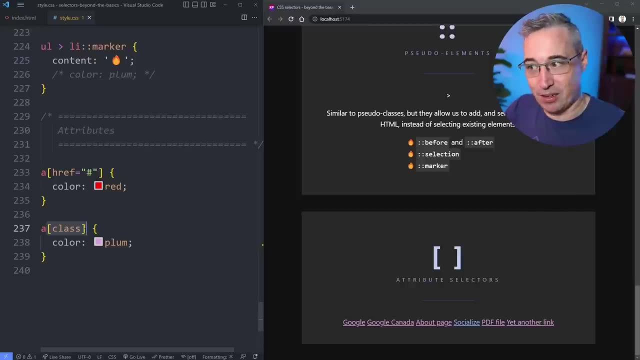 Because I forgot to save my HTML page. There we go, So the socialize is not changing, because it's the only one that doesn't have a class on it. Now, interesting, with the attribute selector You can do this, putting only the attribute, or you can do the entire thing. 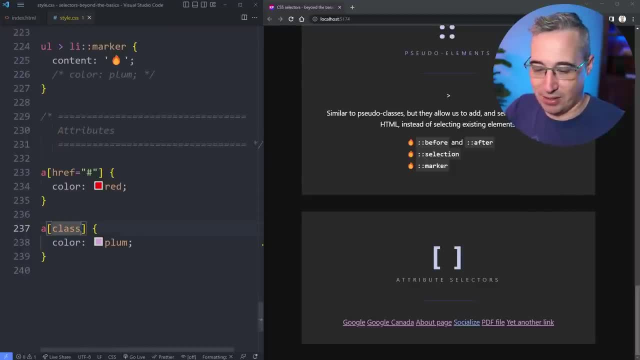 So I could select a class that way, like link three. So I could say is equal to link three, And that would only select the link three, my about page right there. But what I can't do is do something like having it that way.